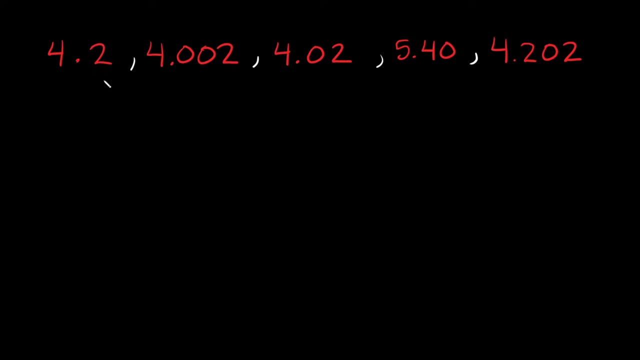 one that stands out as being either the smallest or the biggest. Alright, so we can just look at the whole numbers to begin with. So here we have a 4, here we have a 4, got a 4,. here we have a 5, and here we have a 4.. Okay, so great, I don't. 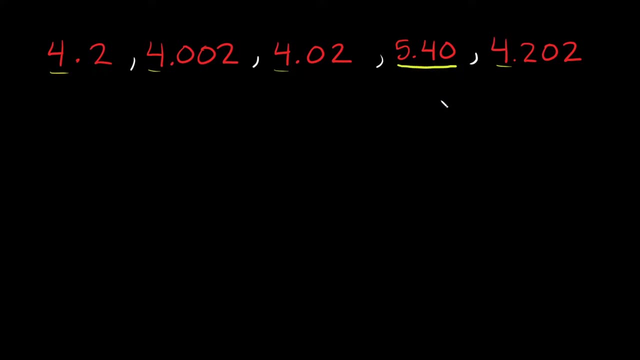 even have to do anything. I already know this is my largest number. How do I know that? Well, because there's a 5 right here for the whole number, right in the ones place. The rest of these have a 4 right. 4 will never be bigger than 5.. So 5 is. 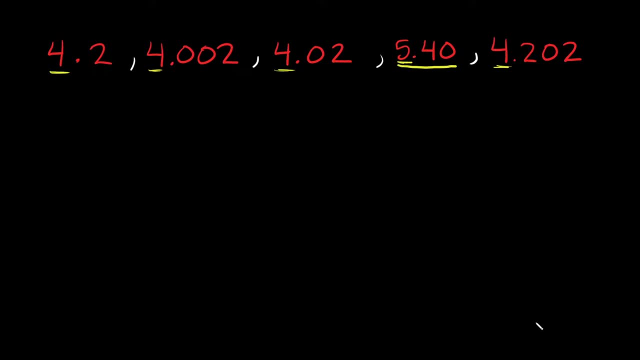 automatically our biggest number, So I'm just gonna write that down here already: 5.40.. Okay, that's our largest or greatest number. Alright, so we're done with this one. right Now, all we have to do is compare these four other numbers, And the useful way of doing that is by 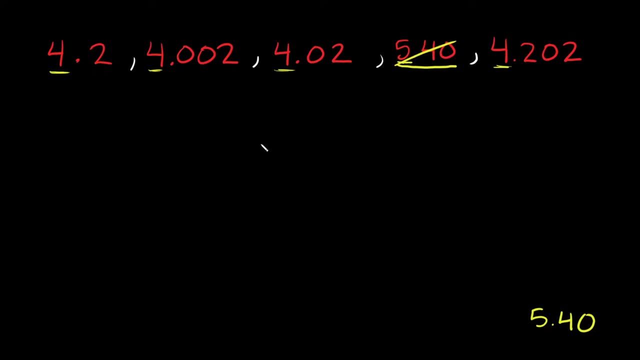 listing them in a column, Okay, but you also have to line them up by their place value. So let me show you what I mean. So first number right here: 4.2. Okay. so I'll just write 4.2. Okay. next number we have here is 4.002.. So I'm 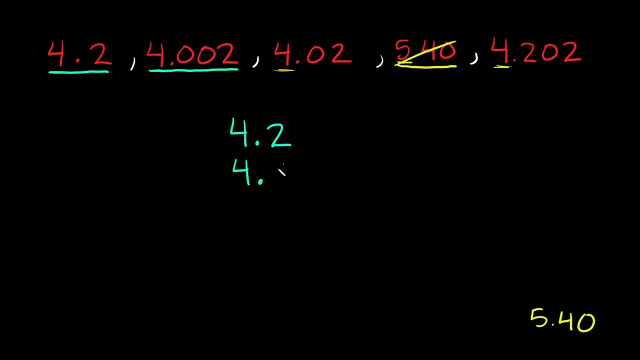 gonna write it right underneath it: 4.002.. Okay, so you see how my numbers are aligned. right, The decimal points are aligned. Now my next number right here is 4.02.. Okay, so 4.02.. And then, lastly, we have this: 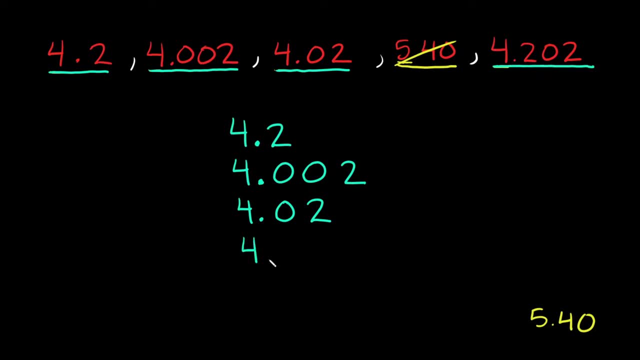 number right here: 4.202.. 4.202. Now, before we start comparing these, one other thing you can do is You see how this decimal number and this decimal number each have this right рес 부분이 are grouped together Because, as you will see, each one of these listen, I'm sad. So for me, for me, if this was, 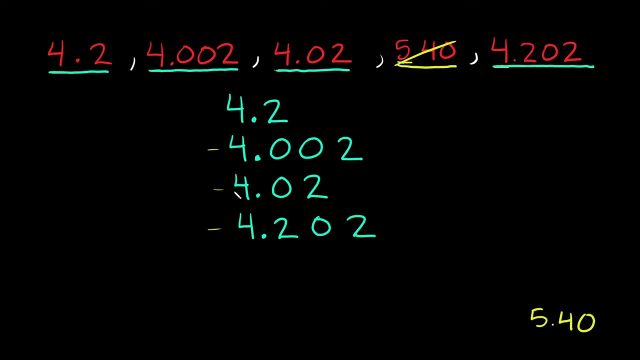 three decimal places and this one only has two and this one only has one. right Now, something that's gonna help us compare these is if they all have three decimal places. okay, So, in order to kind of fill in the gaps, if you will, you can. 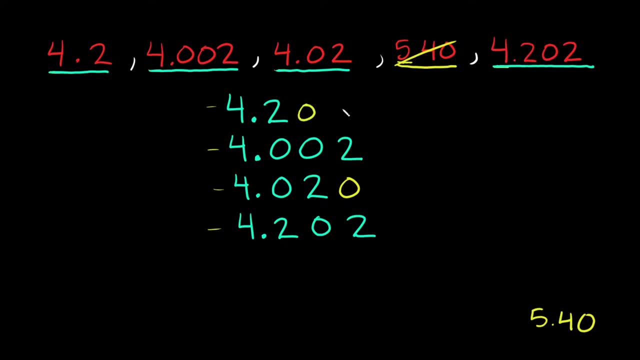 just write zeros there, okay, And I'll write a zero here and here, All right, great. Now they all have three decimal places, right? So now it's gonna be a lot easier to compare all of these to one another. Also the reason I can just add: 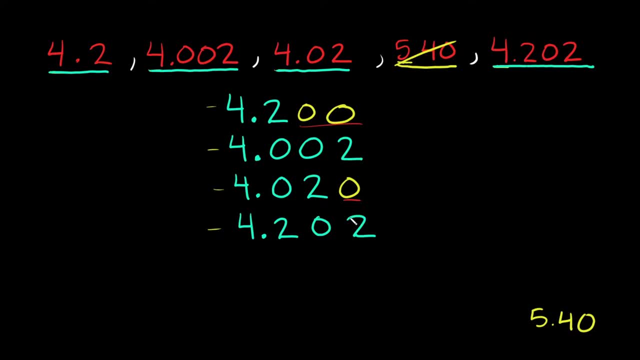 these zeros to the end like. that is because when you add zeros to the end- right, these are at the end of a decimal number- it doesn't change the value of the number. I could have a million zeros over here, right, and go forever, Doesn't? 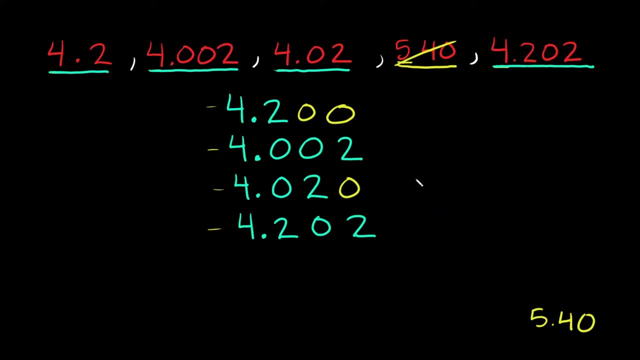 matter, it doesn't change the value of the number, and they are referred to as trailing zeros. okay, So trailing zeros don't change the value of your number. Okay, All right. so now that we got that out of the way, now we can start comparing these. 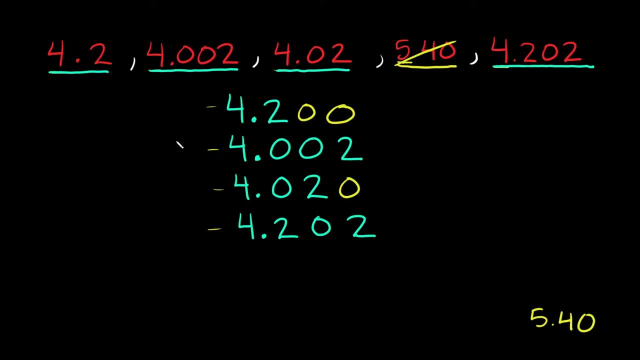 numbers All right. so if we want to list these from least to greatest, we have to figure out which one is the smallest or the least right, And the way we're gonna do that is by going through each of these numbers and comparing one place. 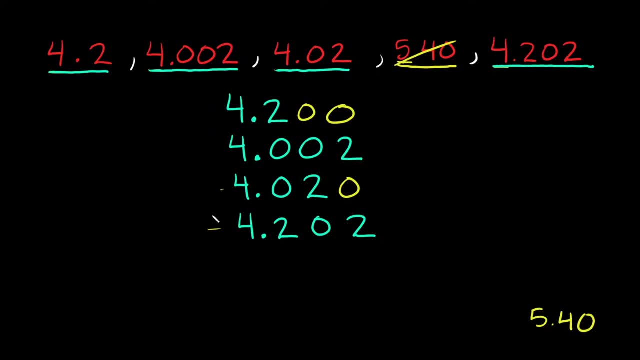 value at a time. So we're gonna start in the ones place and then, if we have to, we'll go to the tenths place, And if that doesn't help us, then we'll go to the hundredths place, And if that doesn't help us then we'll go to the thousands. 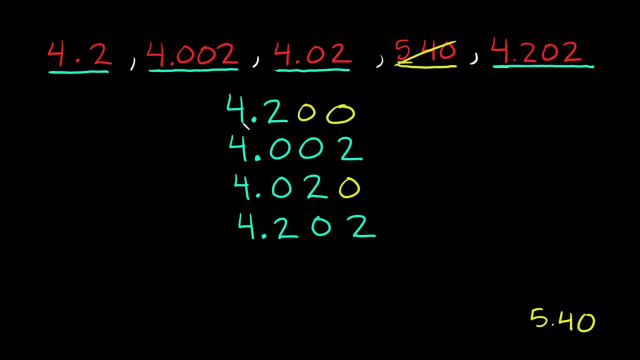 place, okay, And then you just keep going down the line like that. So, starting here in the ones place, you can see that there's just a bunch of fours right. So that doesn't help us. So this is the ones place right. So now we. 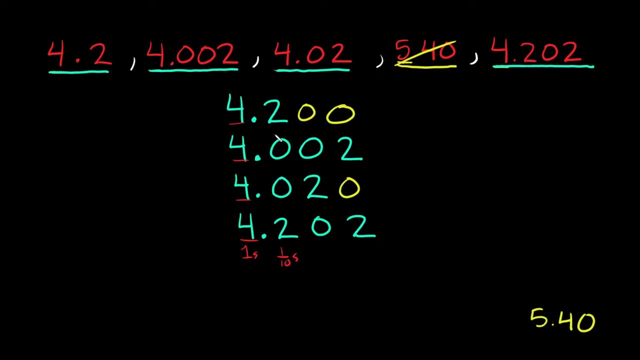 have to go to the tenths place. So now we have to compare the tenths place and figure out which one is the smallest. Well, let's see, we have a two here, we have a zero here. we have a zero here and we have a two here. okay, So, since we have 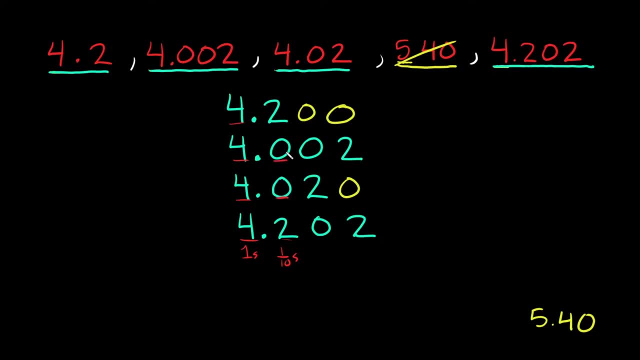 a zero here and a zero here. those are gonna be the smallest, okay? So now we just have to pick between these two, right? So in order to do that, we have to go to the next column, right? So now we have to go to the hundredths. 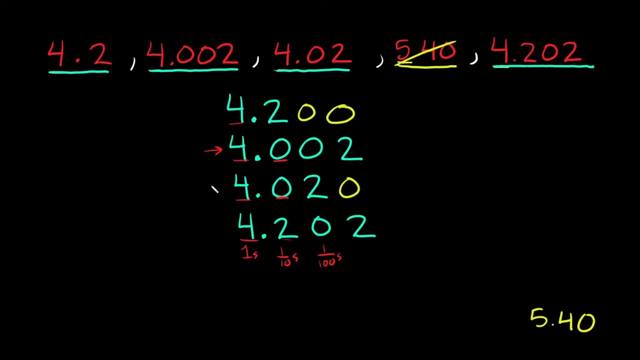 column and compare those. So I'm comparing this one and this one right. So I have a zero here, I have a two here. Zero is obviously less than two, so that means this one right here is the smallest number, 4.002,. alright, So I'm. 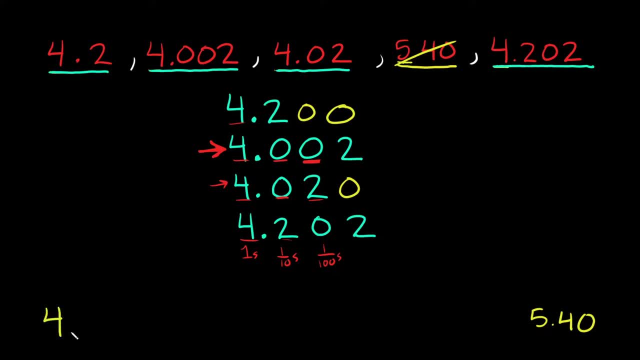 gonna write that down here as my smallest number: 4.002.. Okay, so we're done with this number. Now, which one is the next smallest number? Well, that would be this one, right here, right, Because again, we already went. 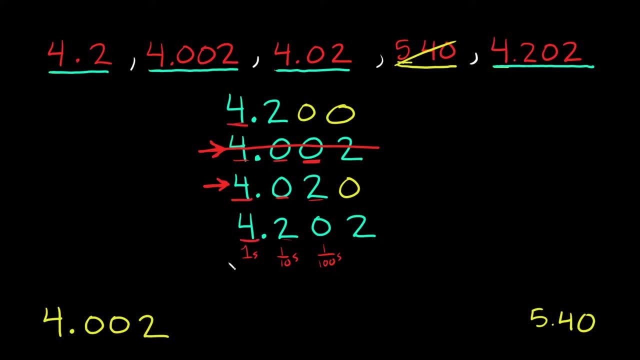 through it. but these all have fours in the ones place. so that means we have to compare the tenths place. So this one has a two, this one has a zero and this one has a two. So which one is the smallest one? This one right here, right? 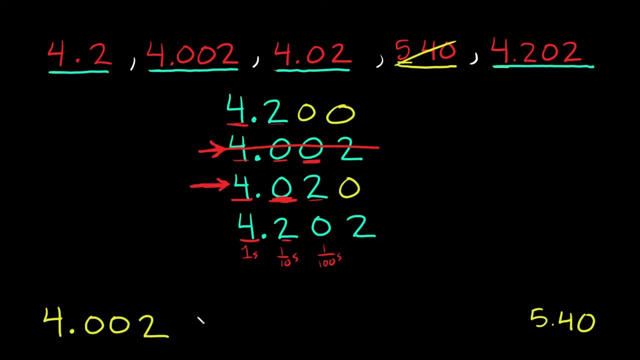 Four point zero, two zero. So I'll write that down here. four point zero, two zero, Alright, great. so now we're done with this one. Alright, now which one is the smallest between the two remaining numbers that I have? So I have this one up here and this: 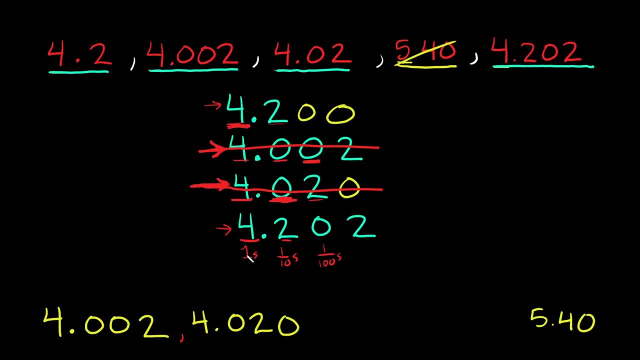 one at the bottom right, Alright, so again. they both have a 4 right here in the ones place, so that doesn't help me. So we again have to go to the tenths place. so there's a 2 up here. there's a 2 up here, Okay, so again. 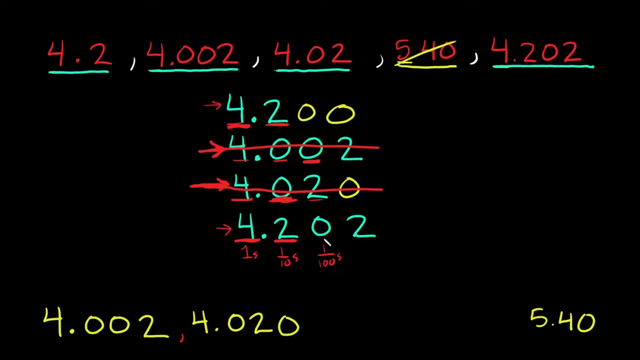 they're the same. so that doesn't help me. So again, I have to go to the next decimal place, to the hundredths place, right? So up here I have a zero and a, down here I also have a zero. So they're still the exact same. so that doesn't. 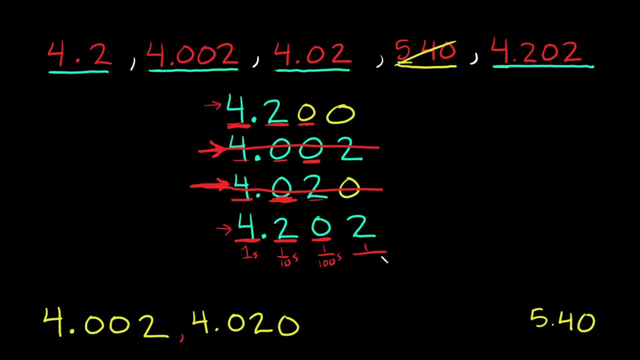 help me. So again I have to go to the next column, to the thousandths place. Okay, so up here at the top I have a zero and then down here at the bottom I have a two. So zero is obviously smaller than two. so that means this one up here is. 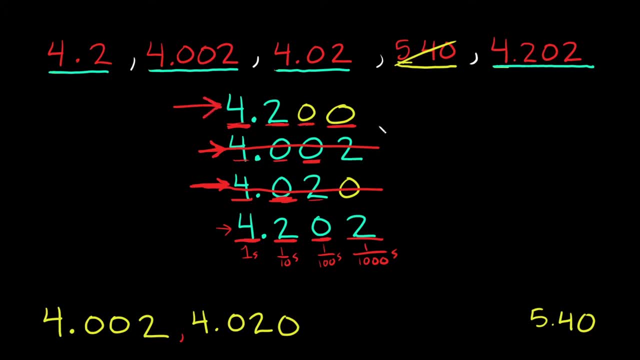 the next smallest. so four point two, zero zero. So four point two zero, zero. But if you remember, I added these zeros in on my own. I only put them there so I could compare them to the rest of the numbers. So actually I can take these out, Okay so, 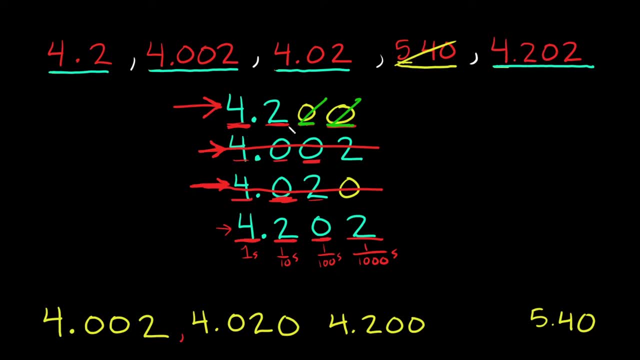 instead of four point two, zero, zero. I really just have four point two. Okay, so that means I can also get rid of these two zeros down here. And also I forgot to do it to the first number. Remember this number right here: four point zero, two, zero. I also added this zero on my own, so that means I can.